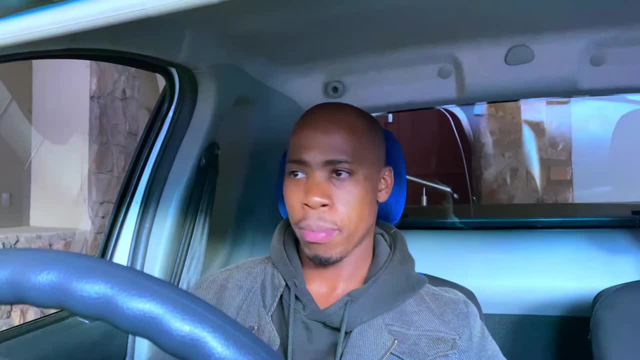 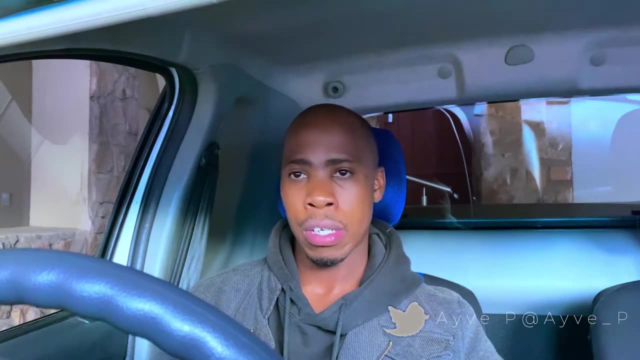 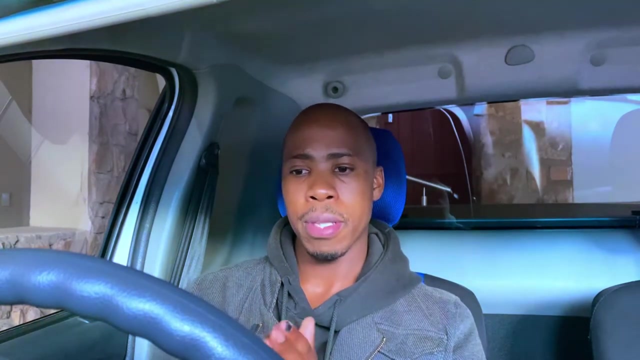 right Or okay. so thermonuclear energy: right, Or thermonuclear power? Well, how does it actually really work? Well, there is, as I said, there is Proton 238, which is essentially used on generators to power and keep warm some of the deep space mission spacecraft. 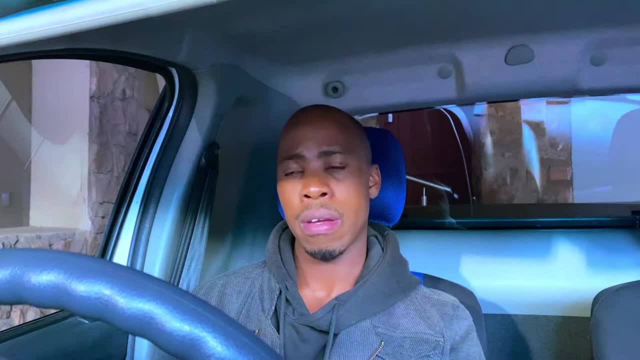 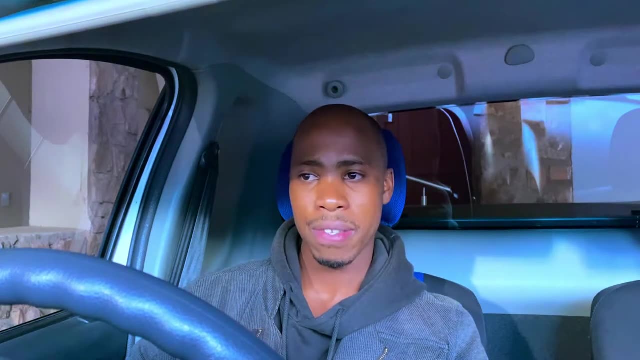 out there. So currently there have been some developments in thermonuclear energy and there is a new kind of thermoelectric energy system right now. that's out there And it's called a dynamic radioisotope power system. And it's called a dynamic radioisotope power system. 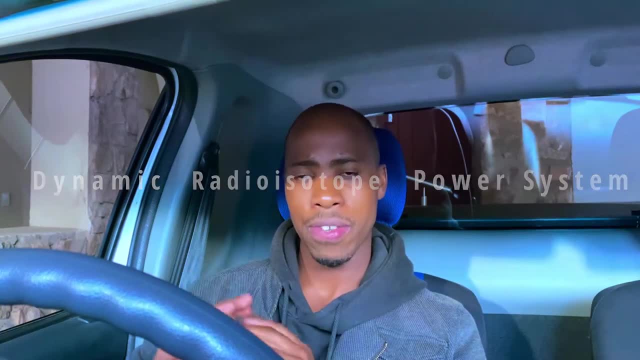 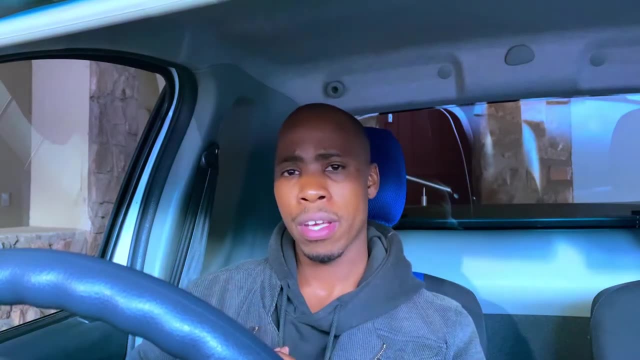 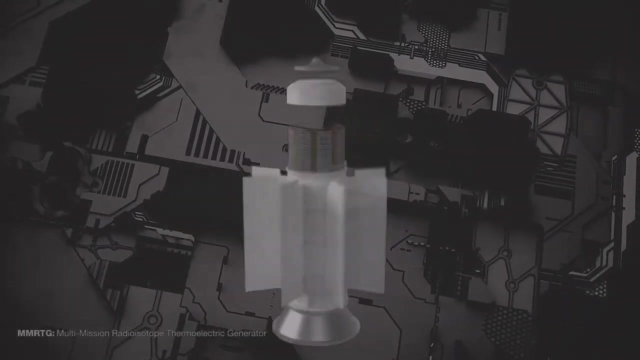 Now, this is a new development and I'll talk about it later on, But for now, let's talk about RTGs first, or multi-mission RTGs. What actually really are they? So let me just quickly show you a quick schematic here. So what you see over here is a multi-mission RTG. This is a typical. 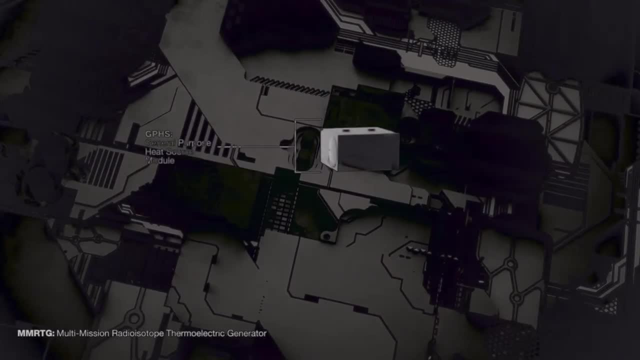 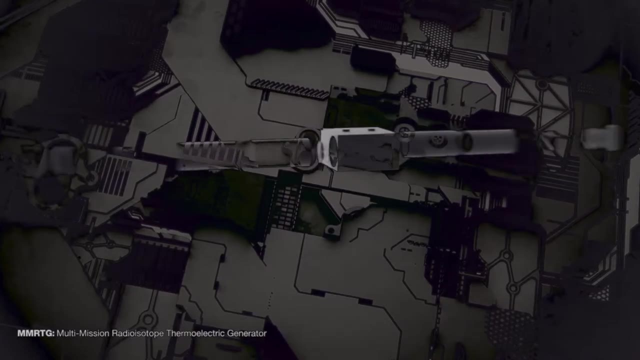 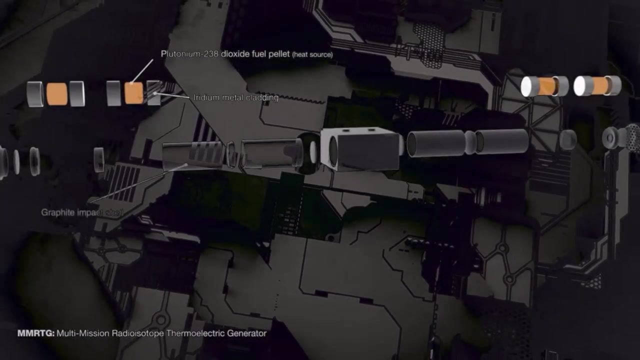 multi-mission radioisotope thermoelectric generator. Here we can see that we have what's known as a general purpose heat source compartment or module. And secondly, we have the plutonium 238 fuel pellets over here. These are the decaying, this is the decaying element essentially. 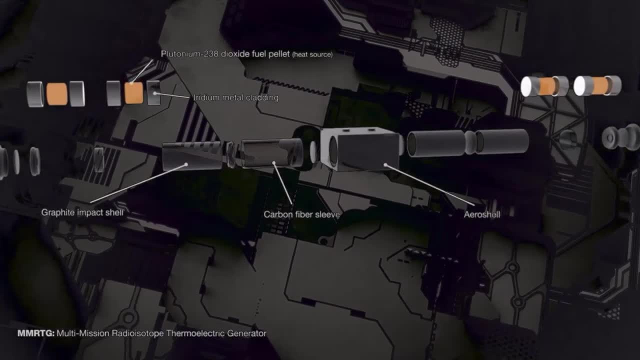 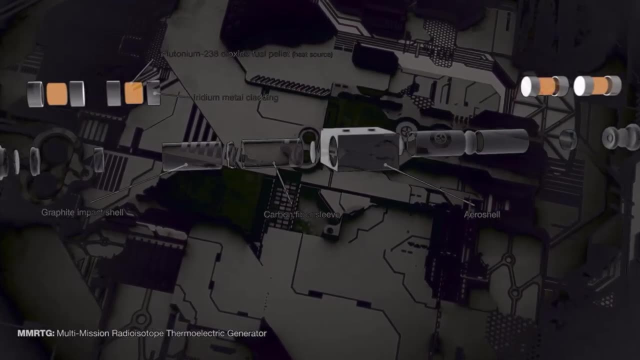 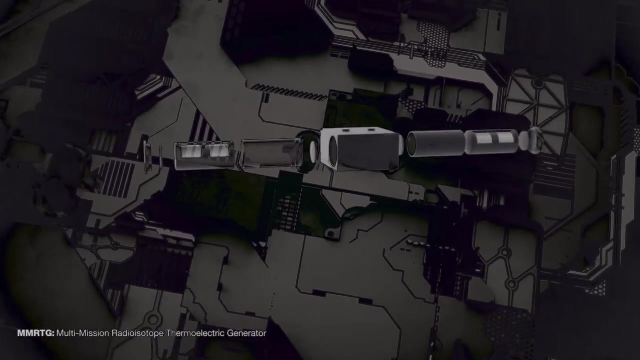 that gives off heat as a result of its decay. So you then have other systems, such as the graphite impact shell, carbon fiber sleeve air shell, and all these are just to essentially ensure that this thing does not get out and harm people. So plutonium 238 is actually very dangerous. You do not want. 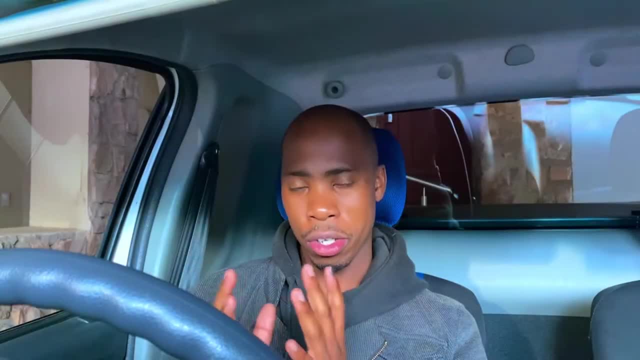 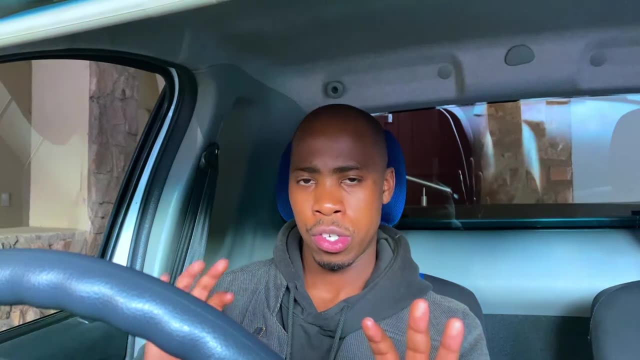 to get your hands on this thing. No, like well, you don't want to get your hands literally on this thing, You want to get your hands on it. But I want to compare RTGs to DRPs. right, The DRP. 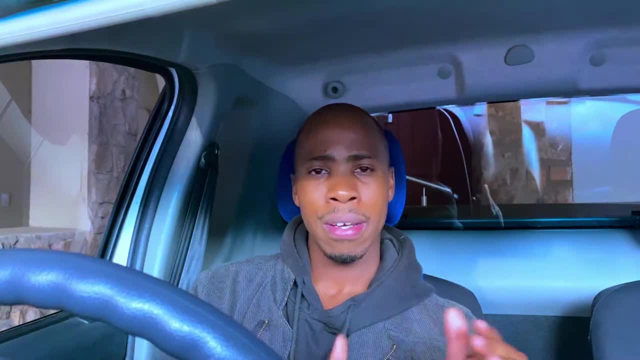 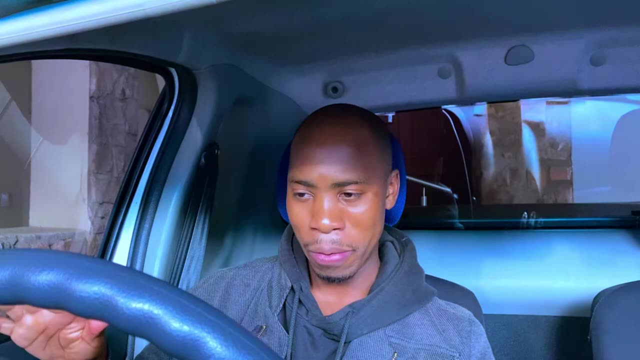 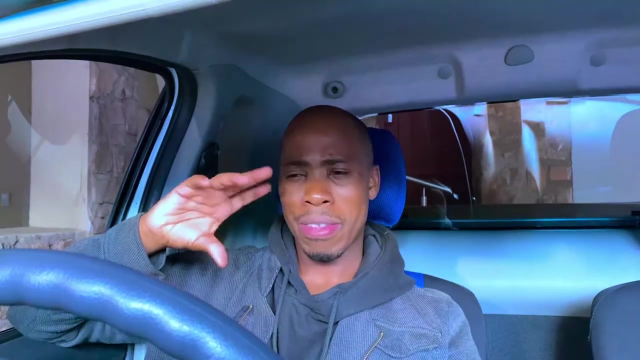 essentially would also be, you know, within that generator system. Now, of course, if you paid any attention in high school you would know a generator converts mechanical energy to electrical energy or does the exact opposite. There are like eight stacks of these, you know, general purpose modules. 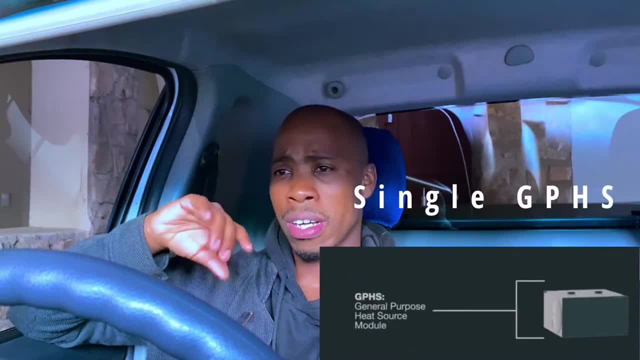 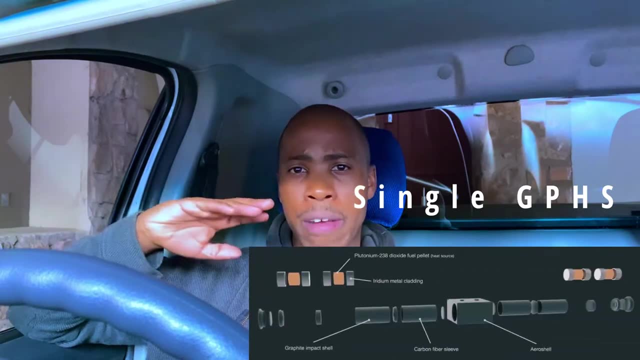 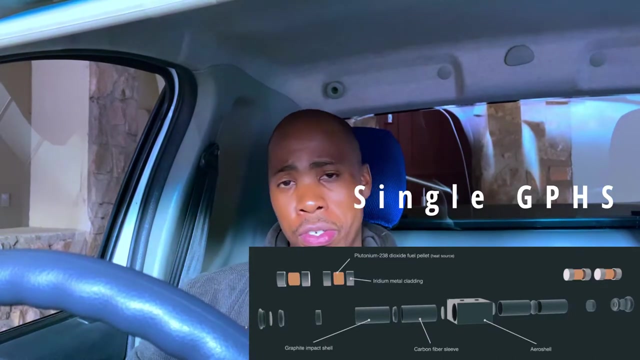 and you know they contain plutonium 238 in there And currently they're just really not that efficient. And the fact that we're also running very low in plutonium 238, the resources that we have in plutonium 238 are actually very low. So how this works essentially is that you 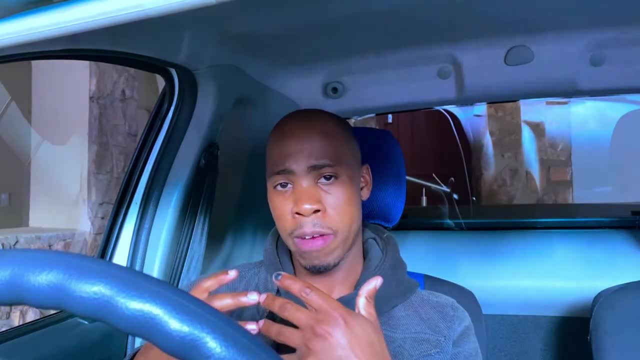 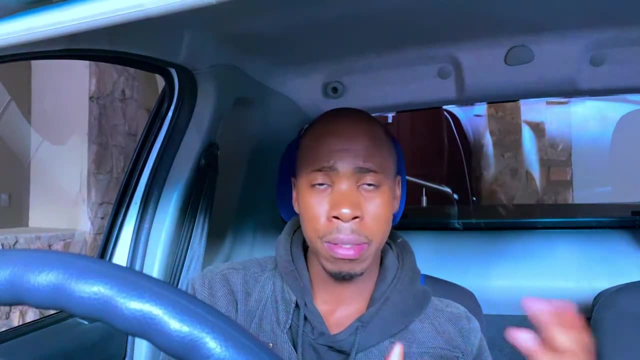 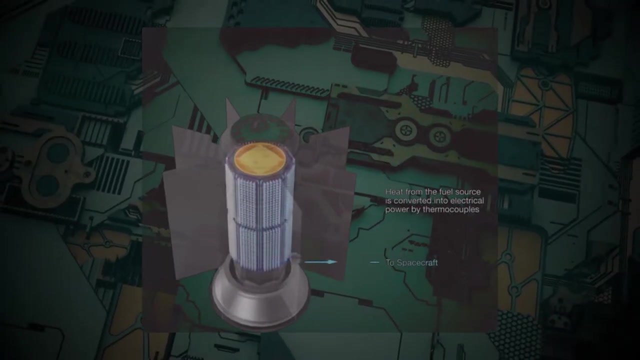 have the heat. the plutonium 238 actually gives off some heat and that heat source, right there from the fuel which is plutonium, is essentially converted into electrical energy using thermocouples. That energy is sent out to the spacecraft and some of the excess energy, or 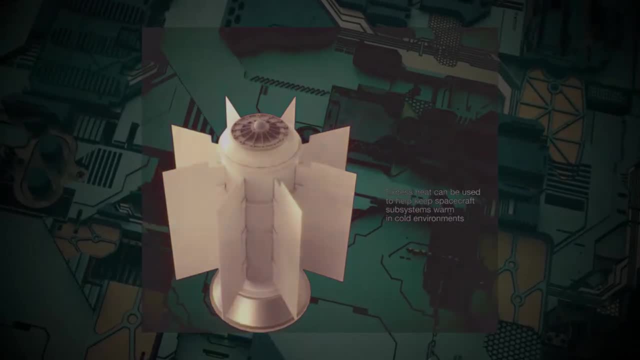 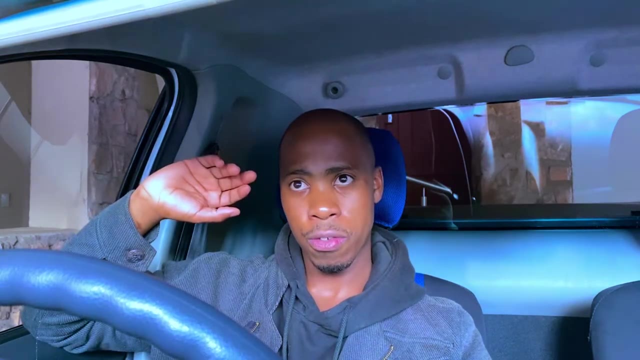 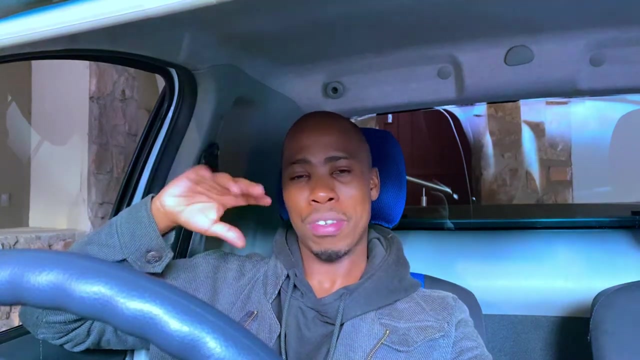 some of the excess heat energy from that is sent out to the surrounding systems And standard RTGs right now, like the RTG that was sent over with the Curiosity Rover, that's essentially not as efficient as it should have been, And this is because it dissipates heat to the surroundings. 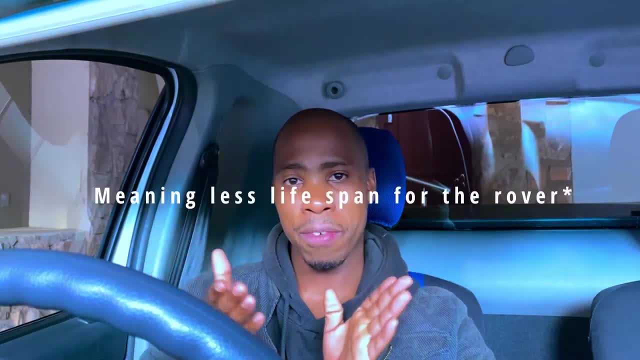 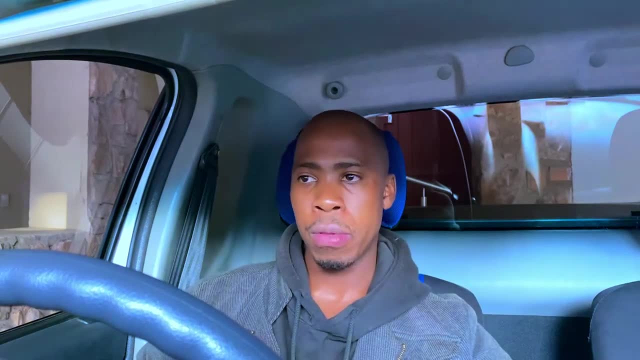 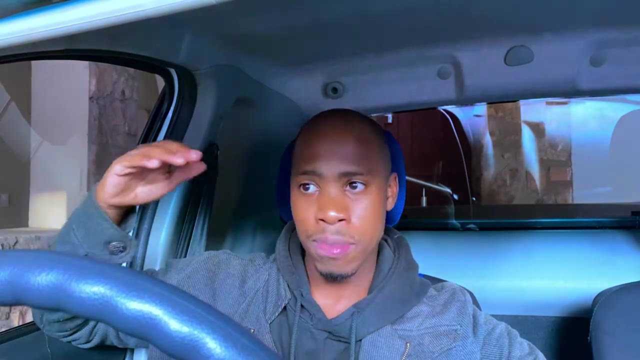 to the surrounding surfaces way faster than it gives off as actual energy, you know, to the spacecraft. So, getting into DRP, So these are, as I mentioned, dynamic radioisotope power systems and these are actually four times more efficient. Right, let me put it this way, For each plutonium. 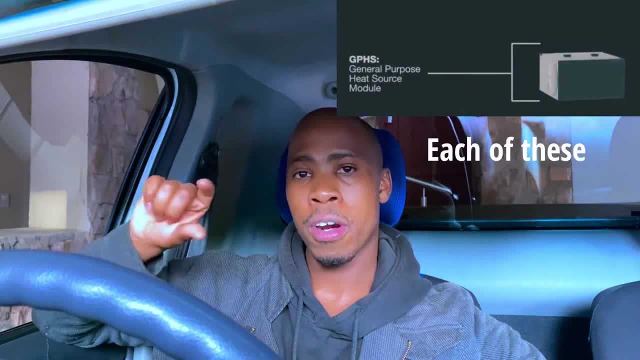 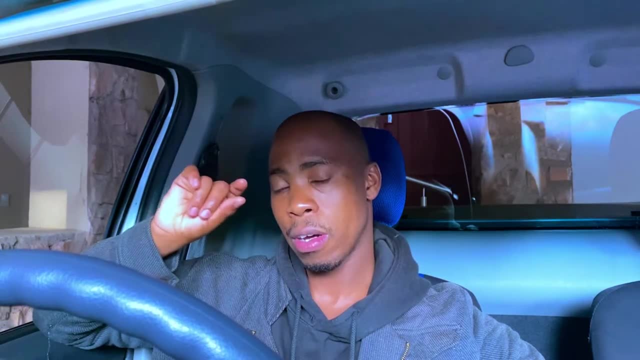 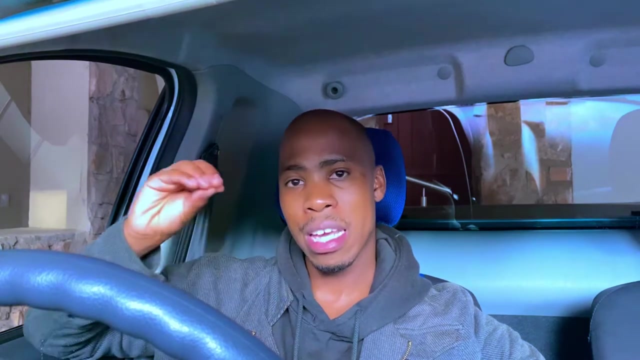 pellet that you have on a standard RTG. DRPS systems provide you four times more energy from that single pellet, right of electrical energy from that single pellet. So what this means is you get four times as much energy from each plutonium pellet source on a DRPS than you would. 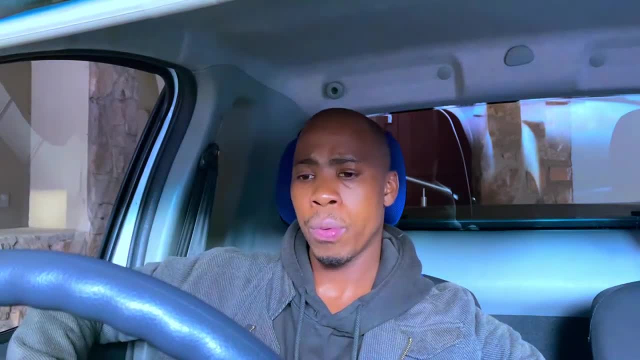 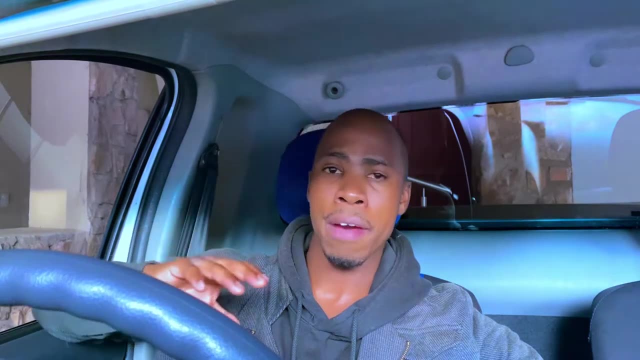 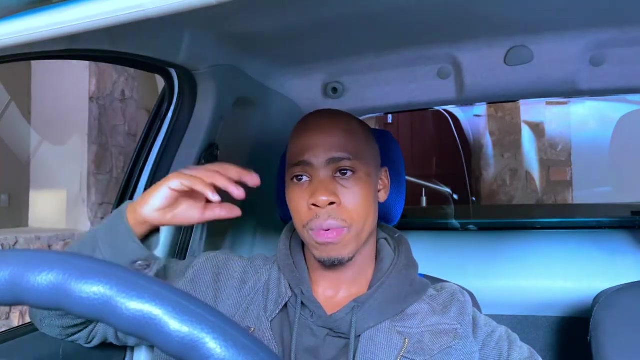 on an RTG, a standard RTG. What this means essentially is that you can stack up less of these modules essentially For the same amount of power you would have on a heavier RTG, Because the more you stack up, the more resources you use, And we need to actually use quite less of these resources. 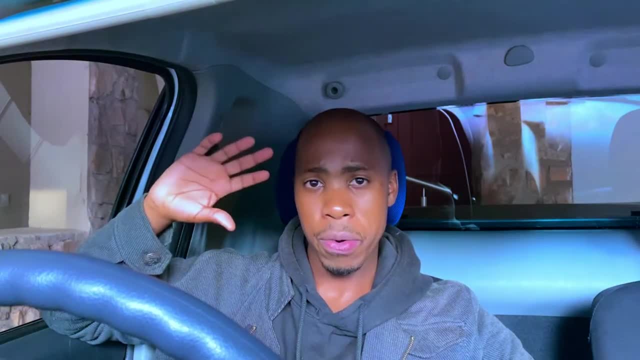 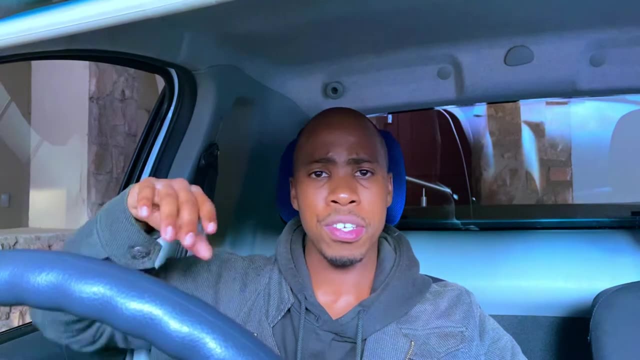 plutonium resources, because we are running out of plutonium. as I said, Plutonium is a very scarce, rare element. Also, the heat dissipation rate for this thing is about half as what you would get on a standard RTG, on a DRPS. So this is huge benefits because, if we're talking deep space missions, like sending stuff to the moon, we want to build a lunar base right now. DRPS systems are better, more equipped. They're more equipped for future deep space missions And these have a proven lifespan of about 14 years. 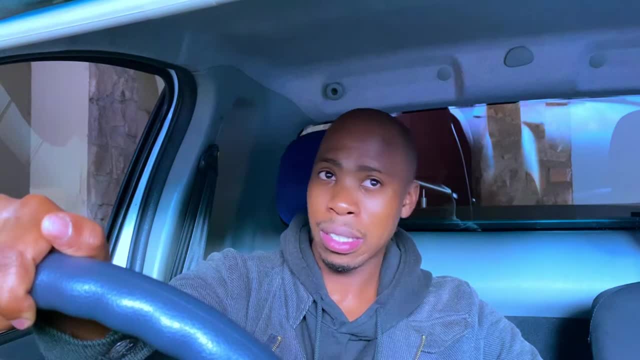 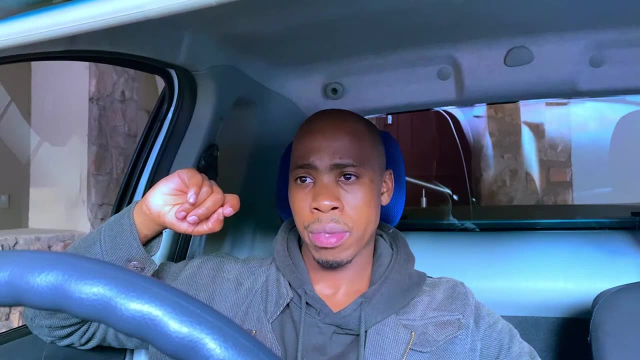 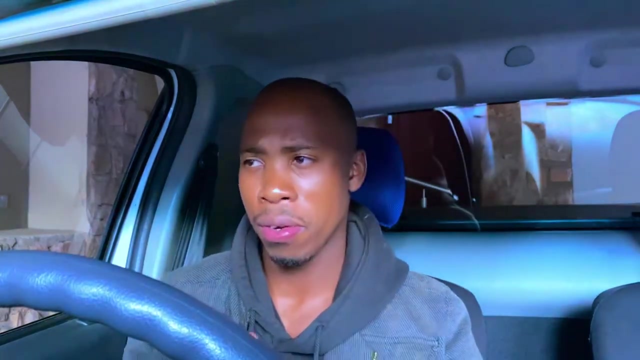 And three years on the ground on Earth. So this is huge benefits actually for deep space missions as well. as you know, now we're talking lunar missions, Mars missions. Okay, so how is the DRPS system better than you know your standard? 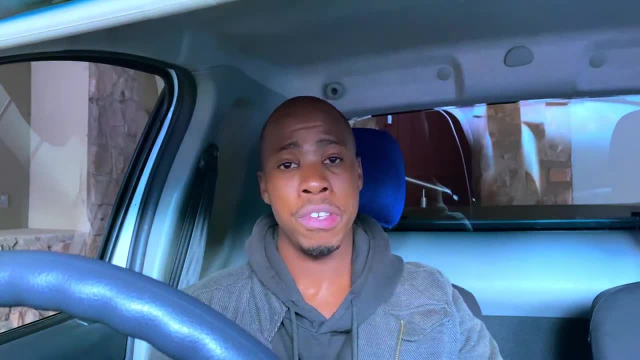 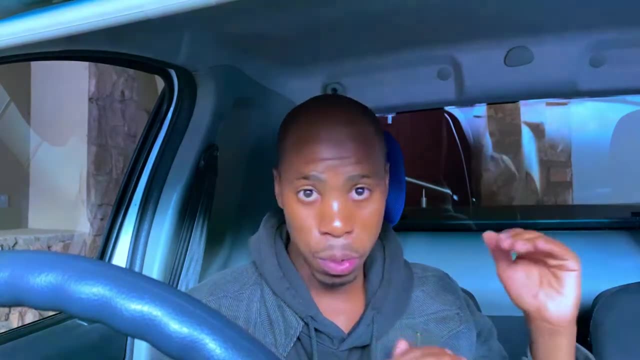 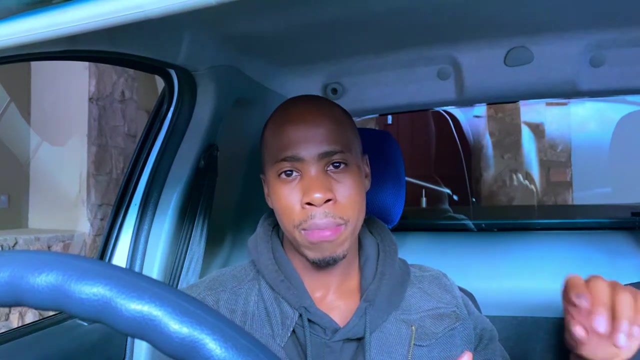 RTG, Essentially on the DRPS system. you can use just six of those GPHS modules to power up the entire spacecraft at full capacity- And I'm talking full capacity- And you can use, you know, two extra as essentially redundant modules. The other thing that makes them way more efficient is 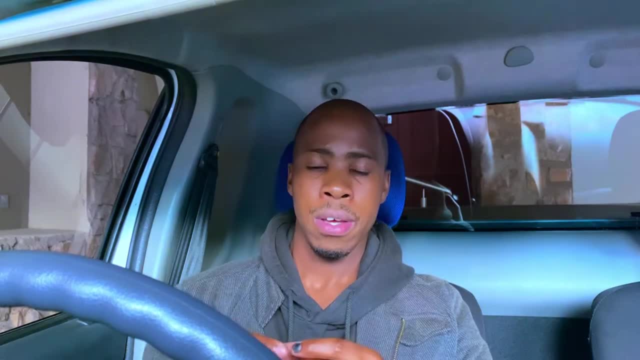 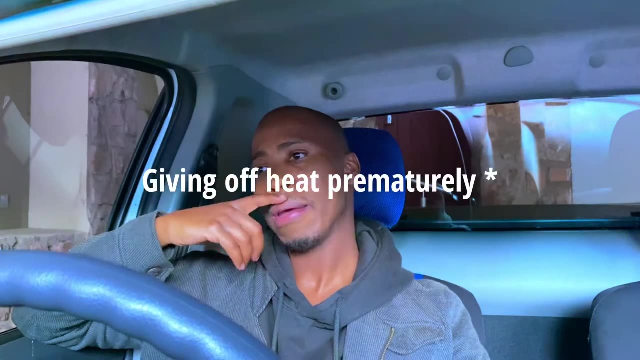 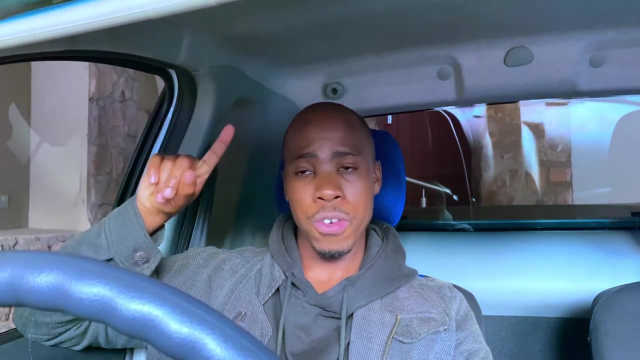 how they're aligned. You actually have a dual opposed alignment here. This prevents the modules from vibrating a lot and hence giving off heat at a faster rate. You don't want any of those ugly things and messy things. You don't have any of those problems actually on a DRPS Also having. 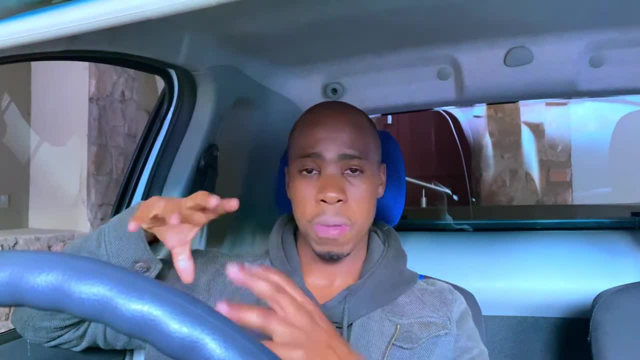 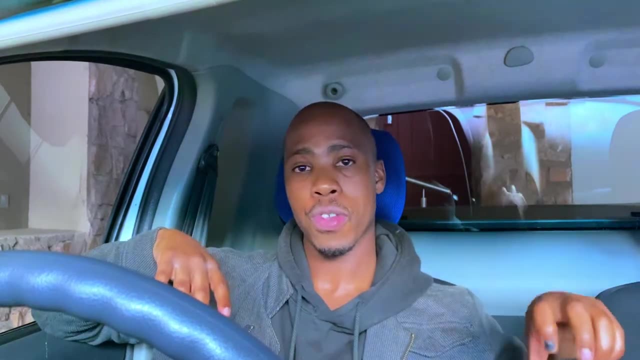 those two redundant modules right there. The GPHS modules are actually more efficient, So you don't have to worry about the GPHS modules. Those redundancies help you still maintain full power capacity. In case two of the six of those modules fail, you still have those two again. You still 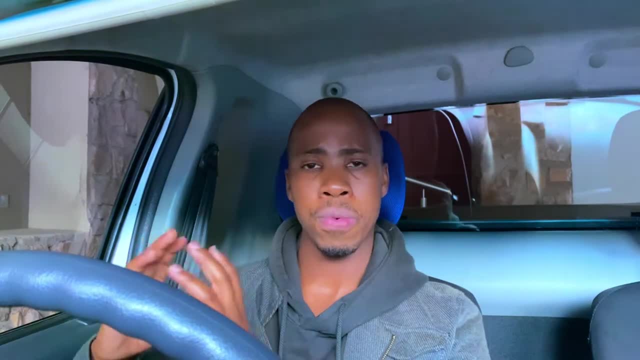 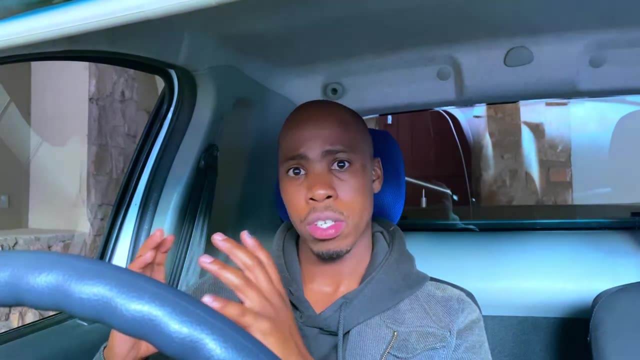 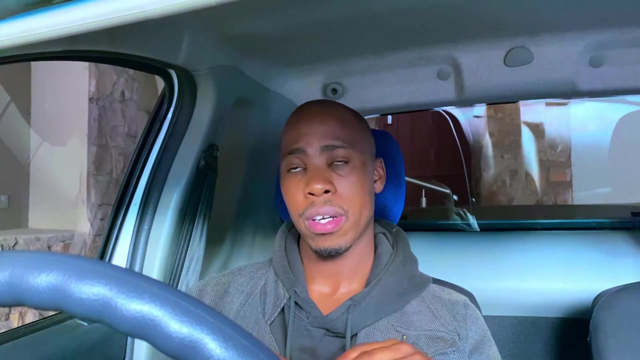 have 100% of the power And if you so, those two redundant modules right there are actually beneficial to you Because, even if you do happen to lose them, you still have your rover or your spacecraft running at full capacity because of the six GPHS modules- GPHS modules that you have. 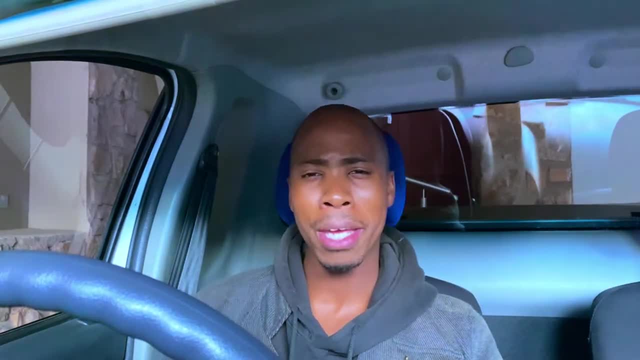 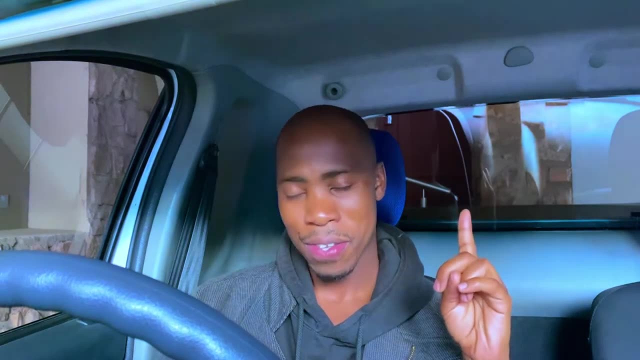 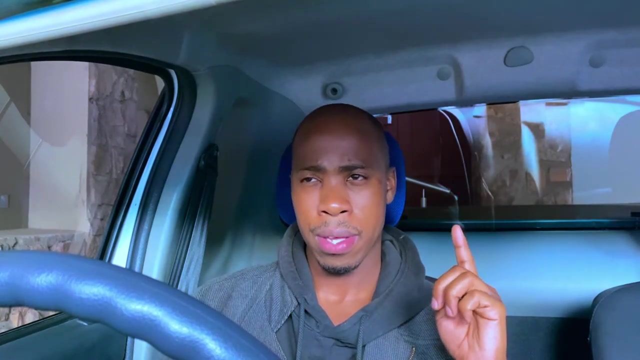 Obviously, you might be asking yourself: well, if this is so great AV, why can't we just use this on cars and bicycles and stuff like that? I'll give you two reasons, Just two. One, this is a very rare substance. Plutonium-238 is not to be, In fact, even Americans used to, I think. 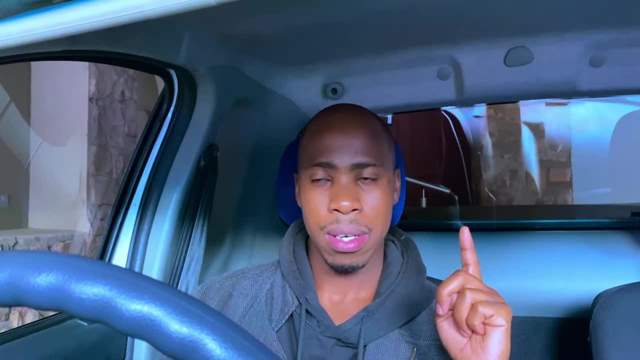 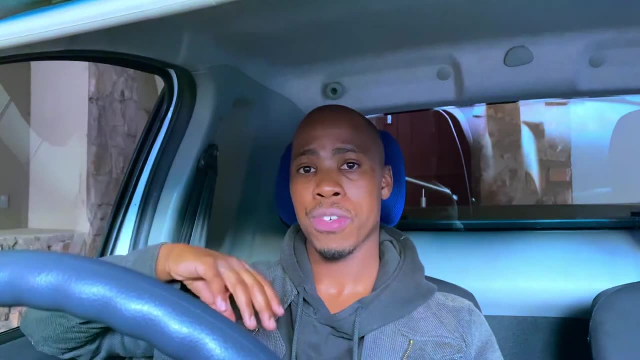 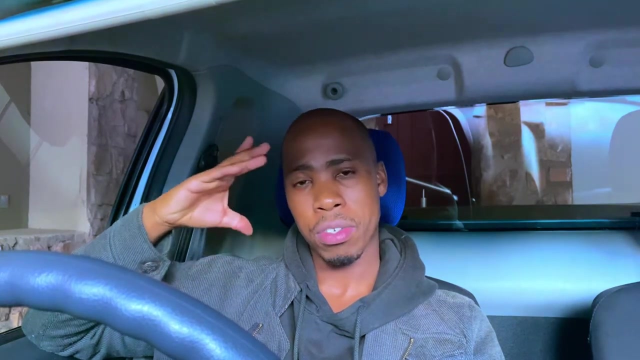 back in the 1970s- I wasn't born then, but back in the 1970s, I think- they used to outsource Plutonium-238 for their spacecraft missions From Russia, and now the entire world is essentially running out of Plutonium-238. But